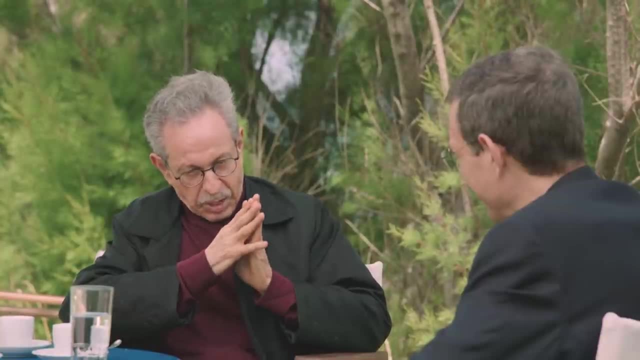 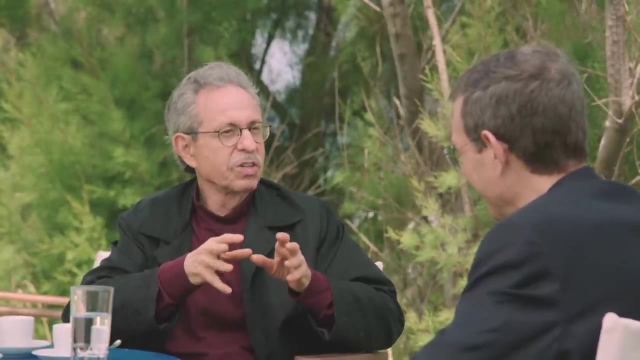 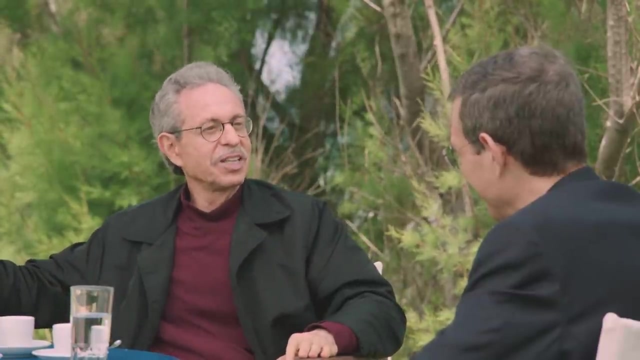 the end what it is, And you've been in a remarkable position. You began in your early part of your career focusing on first stars and the structure of the universe at its very beginning, after the Big Bang, but as the first structure, And you've looked out 10 trillion years to the end. So give. 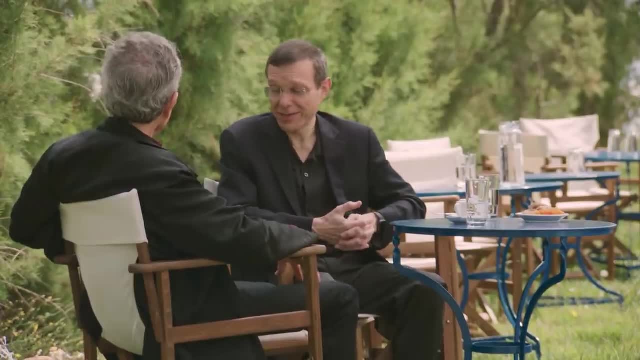 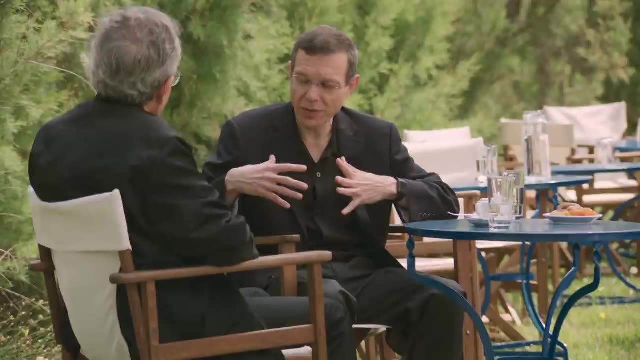 me a sense of the total picture. Yeah, so things started being interesting when the very first stars formed, Let there be light. The universe was getting darker and darker, and then the very first stars lit it up. And then the universe was getting darker and darker, and then the very first stars 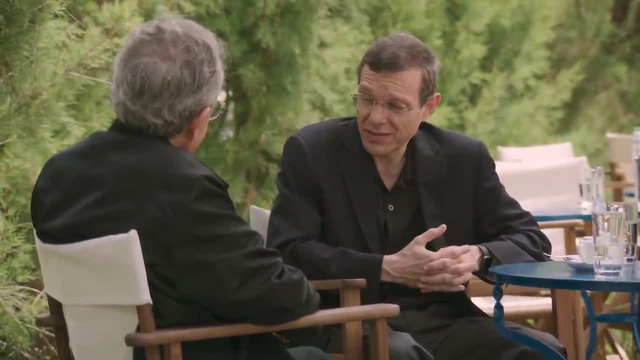 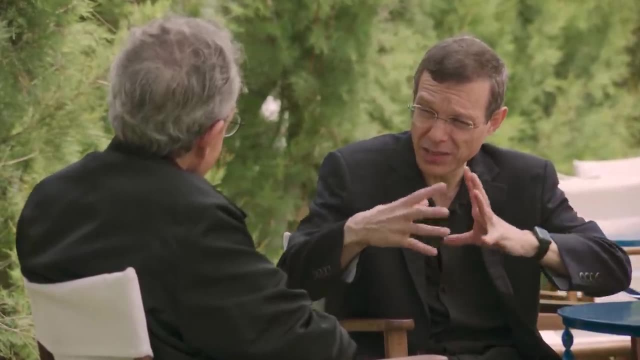 lit it up, And then the very first stars lit it up, And then the very first stars lit it up, And that was 30 million years after the Big Bang. And as time went on, more and more stars formed inside bigger and bigger galaxies, And galaxies like the Milky Way started assembling. 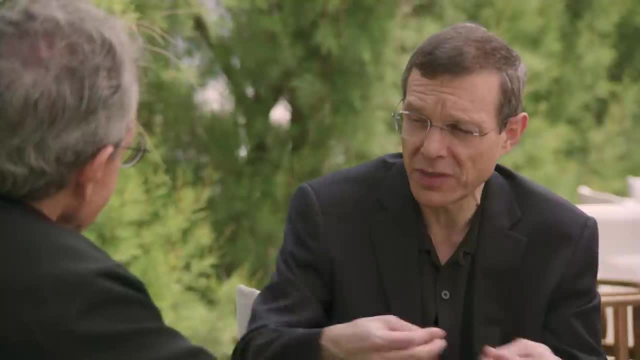 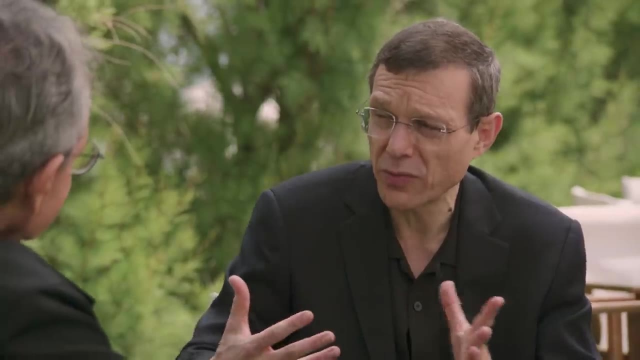 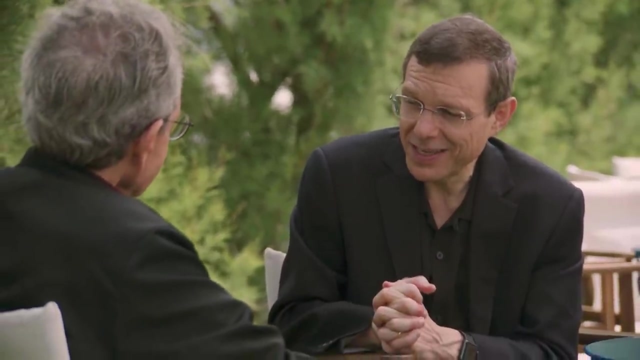 They are sort of midway between the small galaxies that formed early on and the biggest galaxies that formed most recently. The Milky Way formed when the universe was roughly half of its present age, And so here we find ourselves in a galaxy that is sort of typical, inside of which stars like 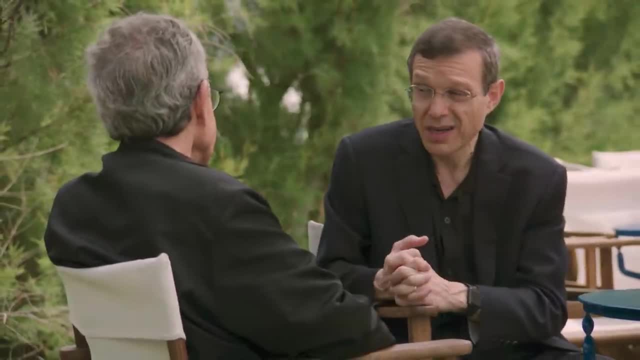 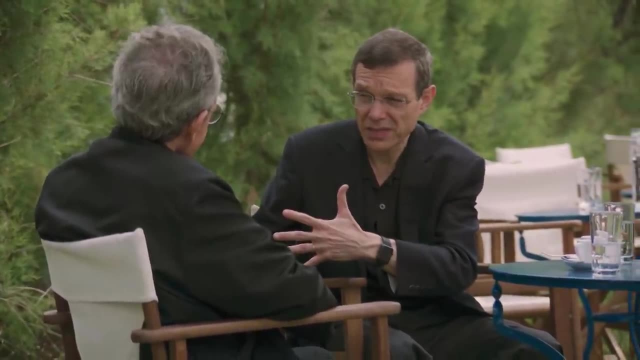 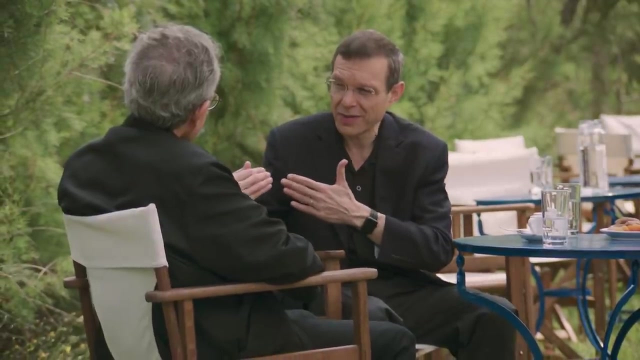 the sun are common, but not the most common. There are lower mass stars that are more common, But at this time in the evolution of the universe, the age of the universe is similar to the lifetime of the sun, which is characteristic. If we were to live earlier on the most, the brightest stars we would have had a shorter lifetime. These would have been more massive stars. The very first stars were much more massive than present-day stars and they had short lives. just like stars in Hollywood, They shine very brightly, but for a short time. And when you say short time, roughly how long The most massive stars, above several tenths the mass of the sun, live for a few million years. Oh, that's very short, because our sun is like 10 billion years. all in, That's right, and And the reason it's important is because these massive stars, if they have a mass somewhere between 8 times the mass of the sun and 25 times the mass of the sun, 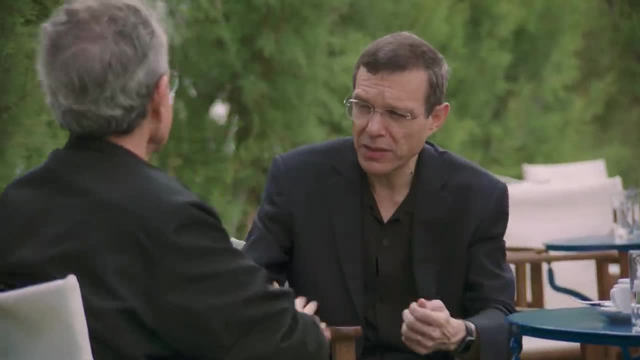 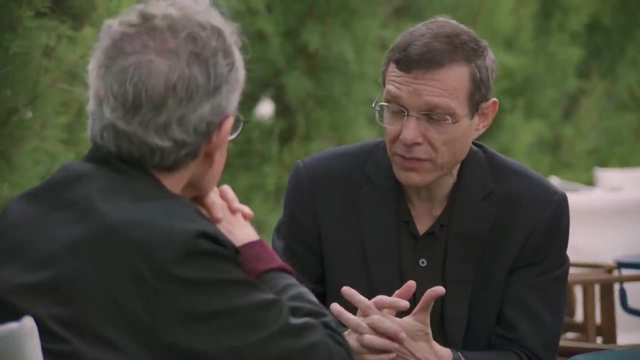 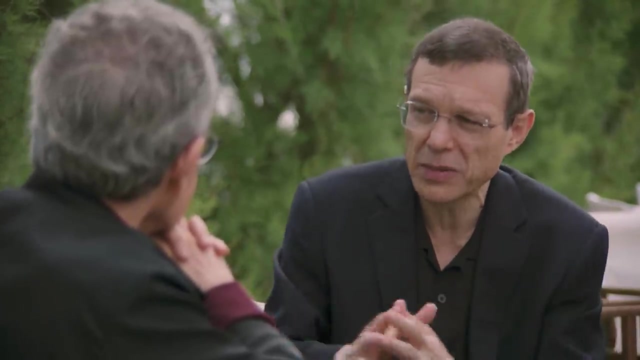 some of these stars explode and they disperse heavy elements into their environment, And without those heavy elements, life would not be possible, because water, for example, needs oxygen, Carbon-based life needs carbon, And all of these heavy elements were produced in the interiors of stars. And later dispersed into the interstellar medium, out of which later generations of stars like the sun, including the planets around the sun, were made. Now, in the distant future, the sun will die and become a white dwarf. It will contract and get its core that will weigh about 60% of the mass of the current sun. First it will expand. First it will expand And Almost engulfing the Earth orbit with its outer envelope, But then its core will contract and cool to a metallic form roughly the size of the Earth. Such an object is called the white dwarf. 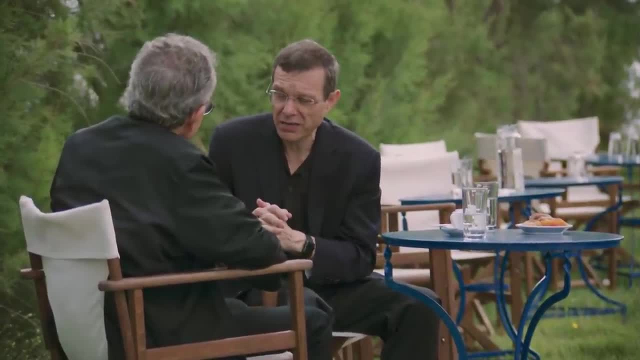 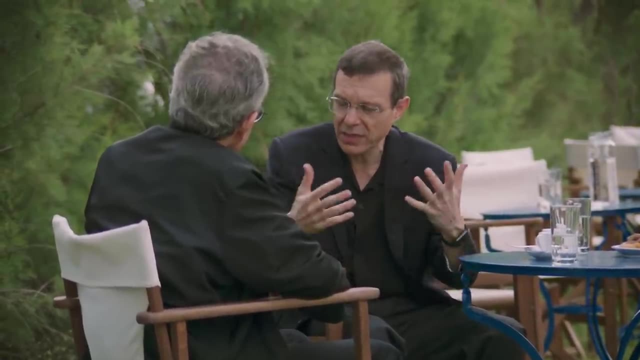 And it will steadily cool into the distant future And the region around the white dwarf will be habitable for a while. But as soon as it cools several tens of billions of years from now, life will not be possible. But as soon as it cools several tens of billions of years from now, life will not be possible. Because when it Chengdu, momentarily, has started toабal in the solar system, we would need to move somewhere else, And the obvious place to move to is then a vicinity of low-mass stars, Dwarf stars that have roughly a tenth of the mass of the sun. They are more abundant than solamente the stars And they are long-lived. They burn their nuclear fuel much more slowly than stars like the sun. They would live up to 10 trillion years And in fact we were trying to find out what's the record lifetime that we can find for a nuclear react. 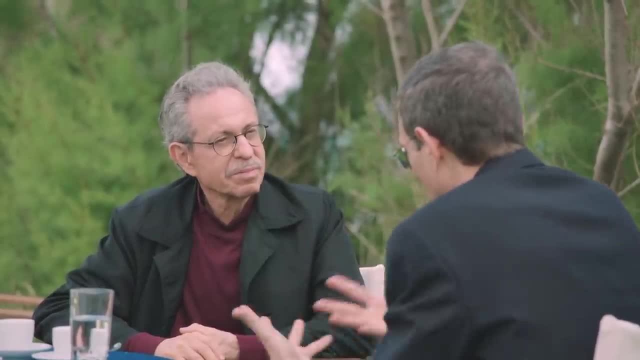 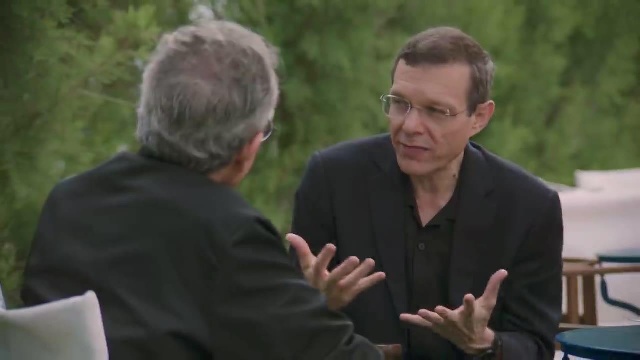 and the Naval orbit reactor held together by gravity, which we call a star. turns out that the hard limit is around 10 trillion years. Beyond that, we would not have these furnaces to keep us warm. We would need to use technology to keep us warm. 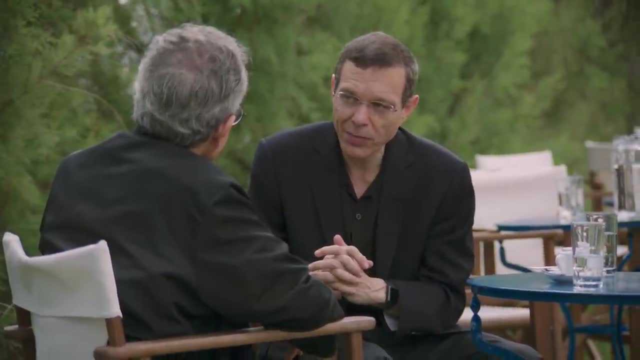 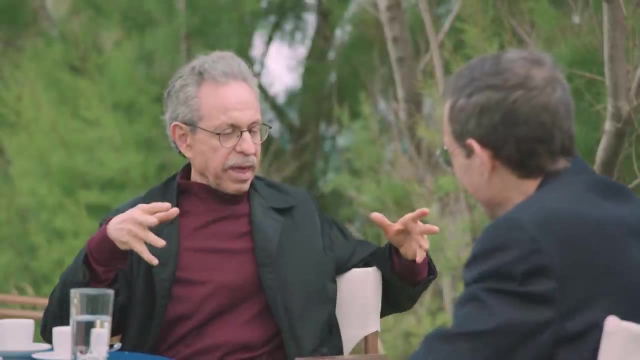 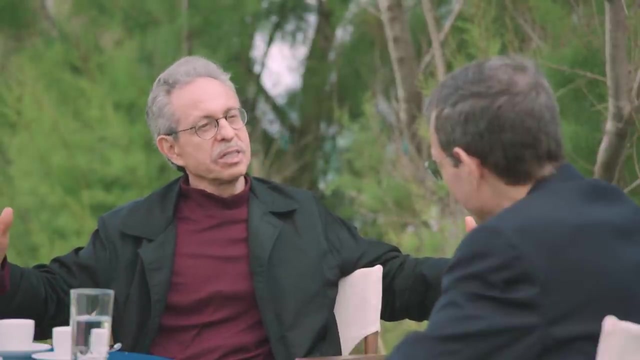 We can have a nuclear reactor that we construct that will keep us warm beyond 10 trillion years from now. For now we have stars. In this period of time, could you classify different epochs? Is there a way, in this 10 trillion year period, can you divide it into segments? 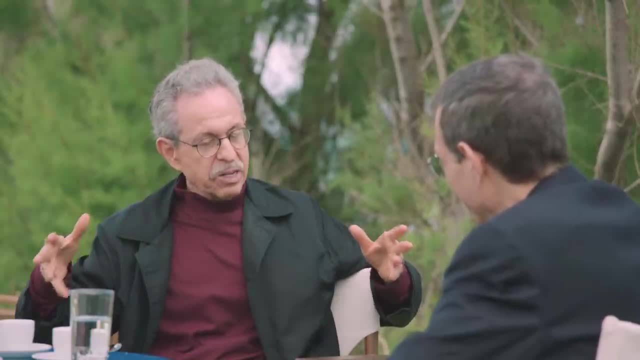 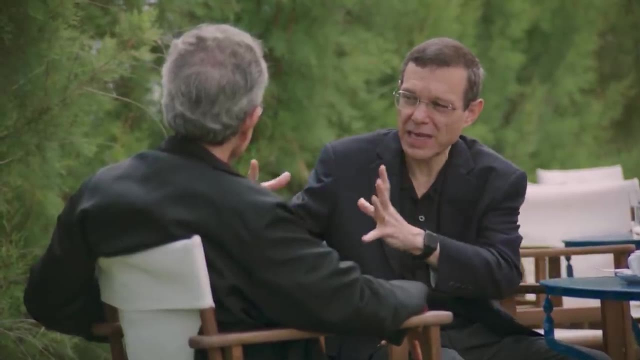 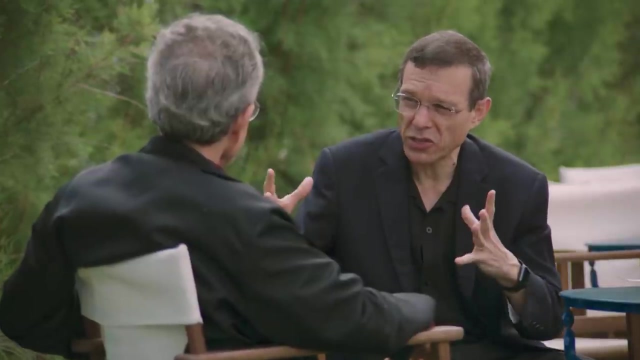 They don't have to be even by years, but even by concept, and we can see how many years in each part just to get a sense of structure. The very first segment in the history of the universe was an epoch during which the radiation 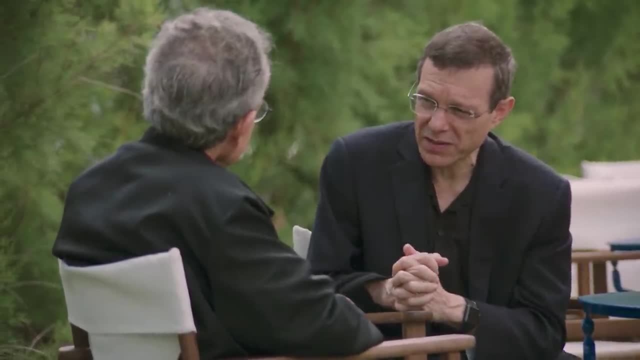 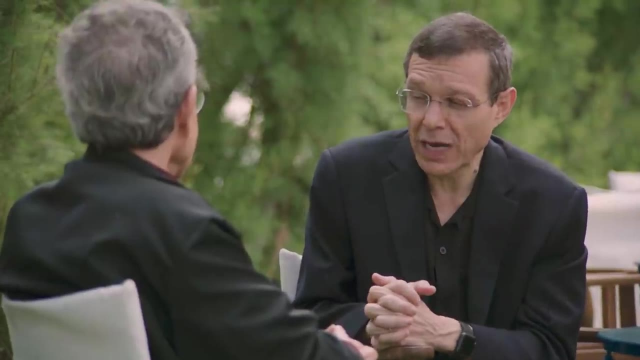 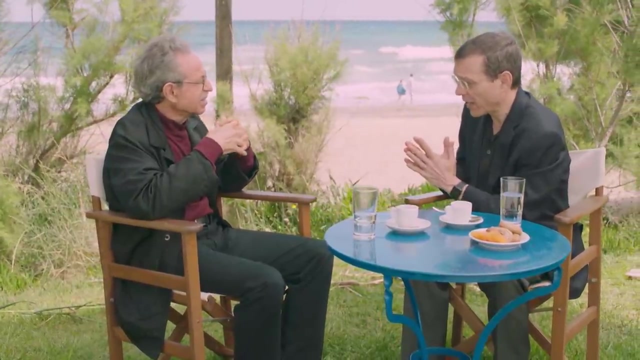 controlled the expansion of the universe. The universe was dominated by radiation, the cosmic microwave background. That lasted for a few hundred thousand years. That was a dark period because you couldn't see through it. No, it was still relatively bright, in the sense that the temperature was above the surface. temperature of the sun, so it was pretty bright. That was the time when radiation dominated the universe. Then, as the universe expanded, the radiation cooled off and matter started to dominate. That's right For a period of order five billion years. 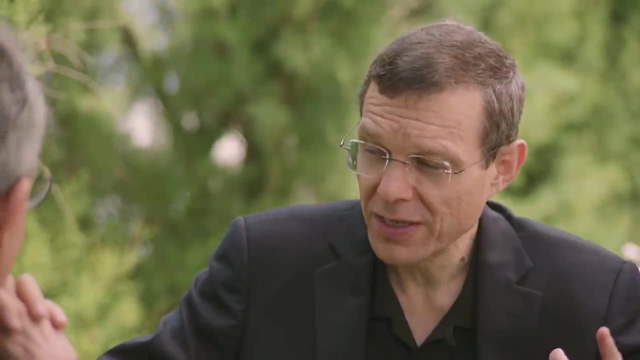 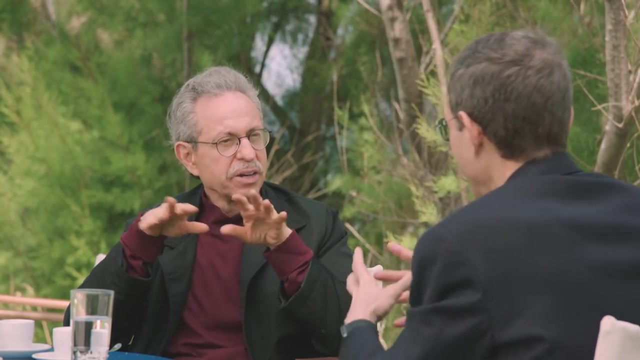 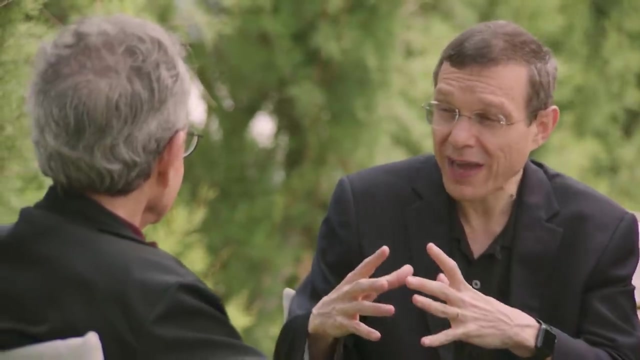 At which point the matter got diluted so much that it became less dense than the vacuum itself, what we call the cosmological constant, The dark energy. that, The dark energy. It's causing the universe to accelerate its expansion. Right, The vacuum does not seem to get diluted like matter. At some point, five billion years or so After the big bang, it was diluted. Yes, Big Bang matter became less dense than the vacuum and at that point in time, the expansion of the universe started to be dominated by the vacuum, and the universe started accelerating. its expansion. That's the epoch that we live in right now. We don't know what will happen in the distant future, but if it continues like that, the future is not very promising for astronomy, because all the galaxies outside of our local region are receding away from us at a rate that keeps increasing with time.